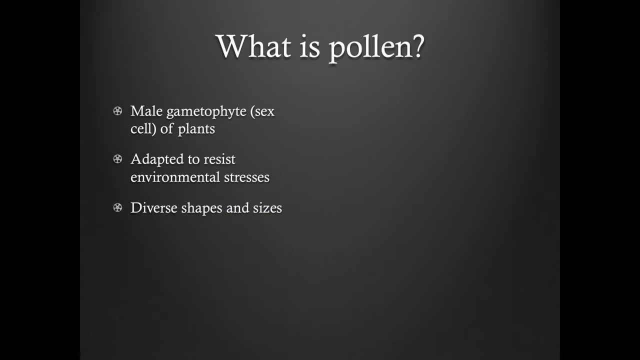 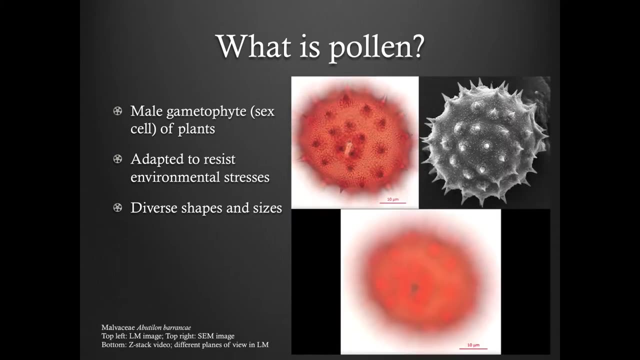 or humidity. Pollen grains can have a variety of diverse shapes and structural characteristics that can help us identify them. Here's an example of a Malvesi pollen grain. The image on the top left was taken with light microscopy. Here is an example of a Malvesi pollen grain. The image on the top left was taken with light microscopy. 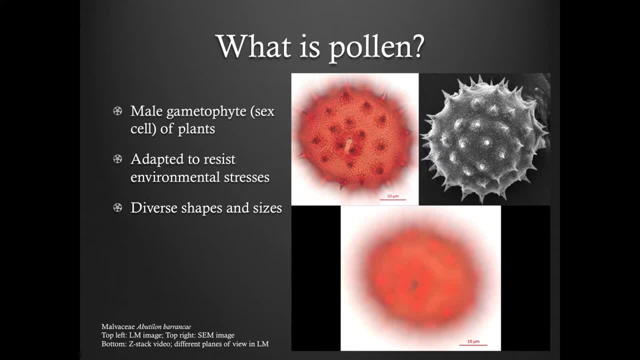 The image on the top right was taken with scanning electron microscopy. On the bottom is a Z-Stack video. This can be a helpful tool for pollenologists. A Z-Stack video is composed of approximately 100 or more images of a pollen grain at varying planes of focus, combined to provide a 3D representation. 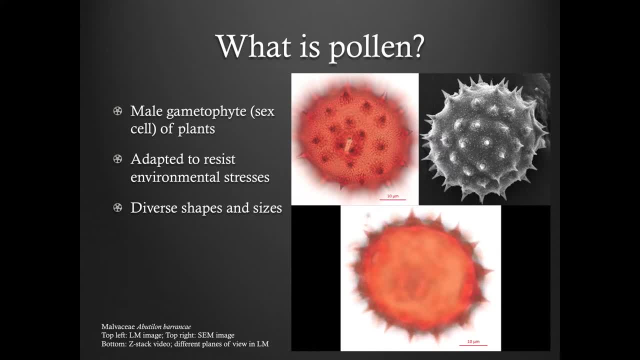 of the grain. This gives the user the ability to look at the pollen grain as if they were looking at it through a microscope. The image of theidorum serves as an 더� Subst. 5. Pollen Grains- Model 6. 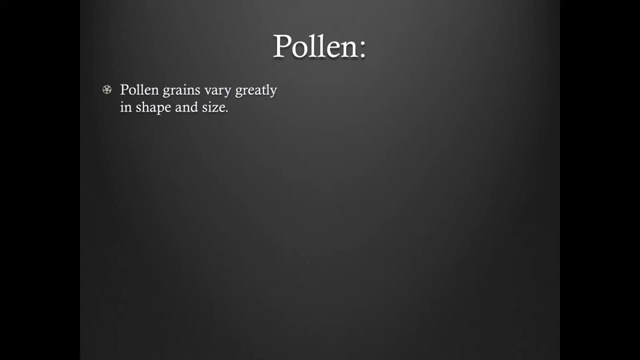 Pollen grains vary greatly in shapes and sizes. Light microscopy images provide a two-dimensional representation of the grain. Z-Stack videos and SEM images can help the user visualize the three-dimensional shape of a pollen grain. A rozum of the dinobacterium's net crust-or-brstatumENT bosses, the formation of this gran accentuates. 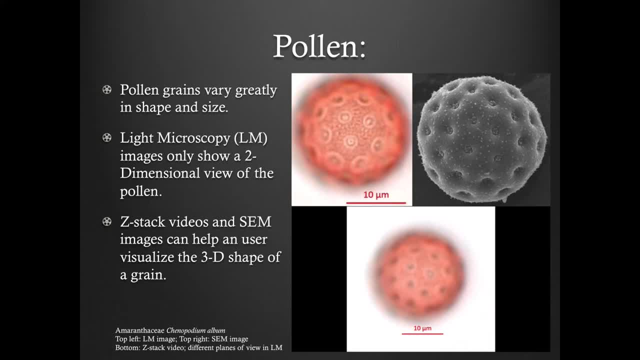 the grain. Use HilloPoller for sampling performance. Here is another example. This is an Amaranthaceae pollen grain. The image at the top left was taken with light microscopy. The image at the top right was taken with scanning electron microscopy. 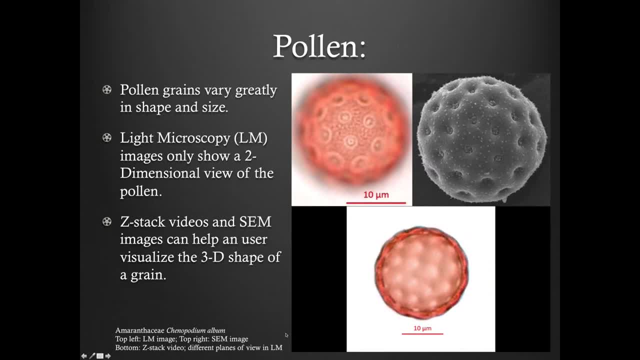 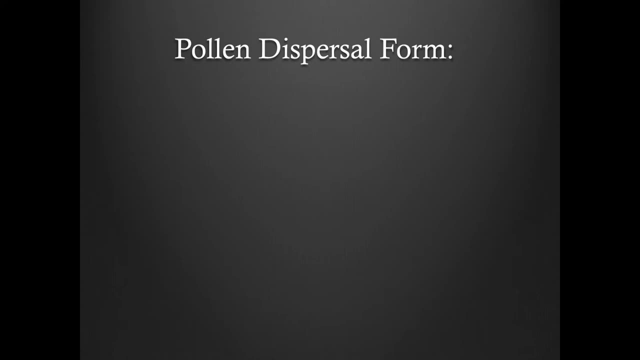 Below you can see the ZStack video. Videos such as these can help the user gain a better understanding of the morphological characteristics of the grain. Fallen grains generally develop as a formation of multiple cells on the anther of a plant. As the grains mature, they may then be classified into different dispersal types. 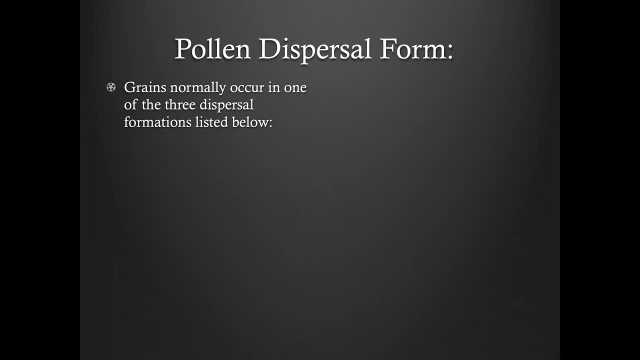 Grains typically occur in one of the three types of dispersal formations listed below. Monads are single cell pollen grains. Here's an example of a monad. Tetrads are pollen grains comprised of four cells. Here's an example of a tetrad. 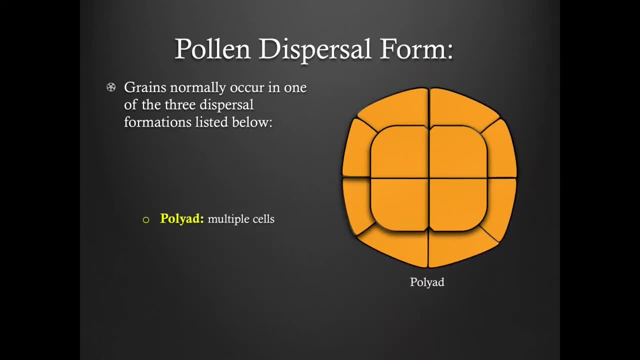 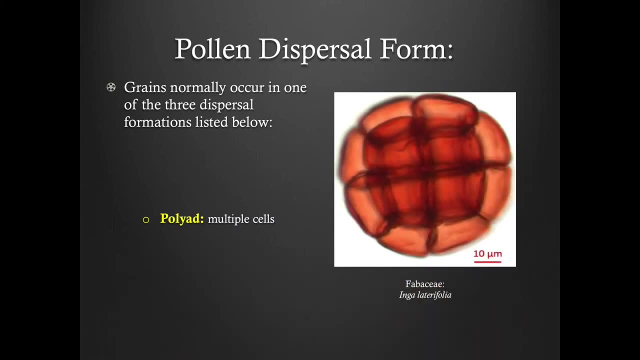 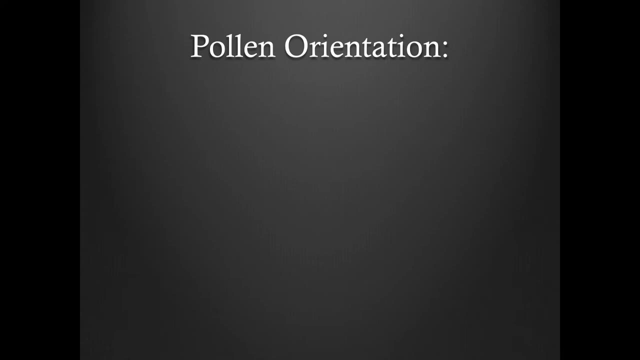 Polyads consist of more than four cells. Here's an example of a polyad. Now let's talk about how to properly identify a pollen grain's orientation. When looking at a pollen grain, researchers need to be able to understand and identify which angle of the grain they are seeing. 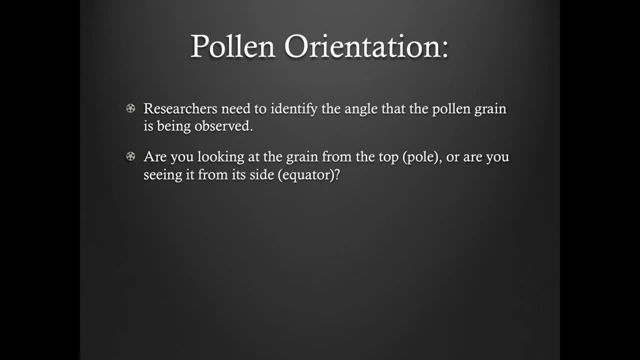 Are you viewing the grain from the top or bottom, which are considered to be the poles, Or are you seeing the grain from the side, which has the equator visible? Those orientations are known as polar and equatorial. To help better understand polar and equatorial orientation, let's use the example of an 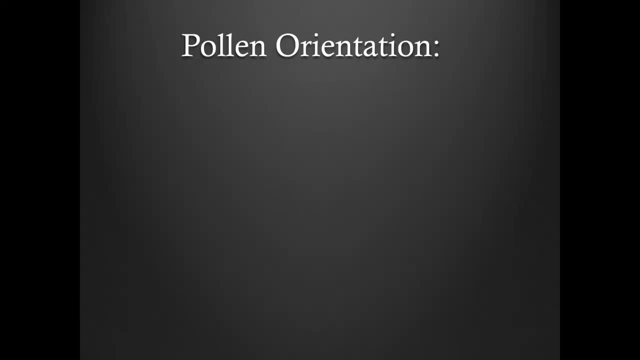 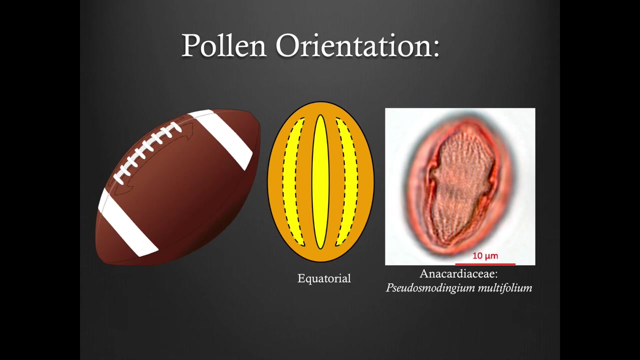 American football. Imagine holding a football in a position where the lacing is directly visible. If this football were a pollen grain, this would be an equatorial view. In the center of the screen is a cartoon representation of an equatorial view. To the right is an anacardiasis grain in its equatorial orientation. 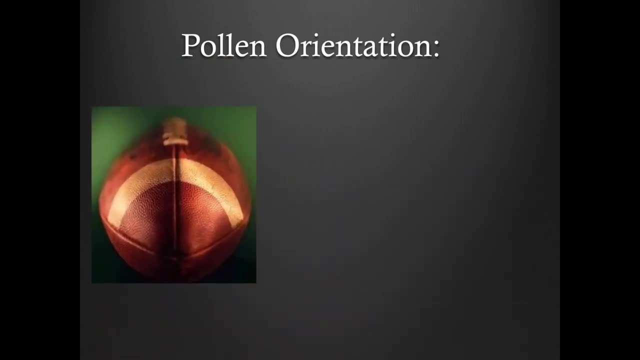 Now imagine holding a football so that you are looking directly at the end. This would be a polar view. In the center of the screen is a cartoon representation of a polar view. To the right is an anacardiasis grain in its polar orientation. 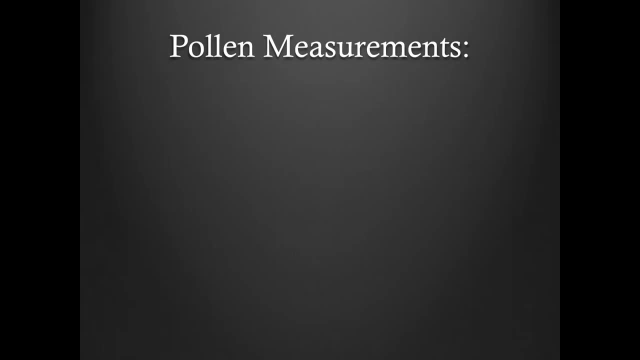 Okay, Now let's discuss pollen measurements. Measuring a pollen grain can provide useful information. When measuring a grain, you need to take into account its orientation. Both polar and equatorial measurements can be done while the grain is in its equatorial orientation. 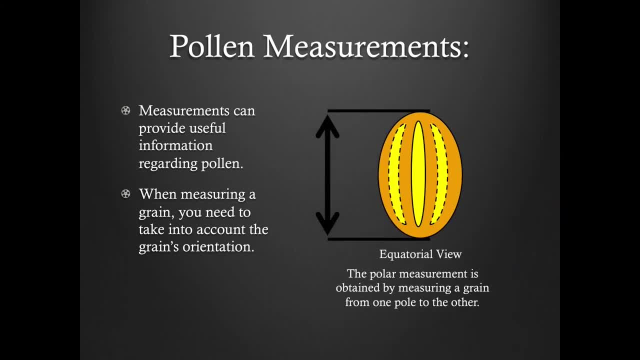 For the polar measurement, the grain should be measured from one pole to the other. For the equatorial measurement, the grain should be measured across the equator. Remember, be careful when measuring your pollen grains. You cannot get a polar measurement from a polar view.